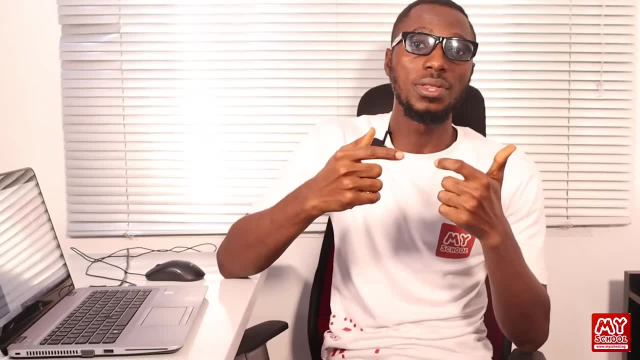 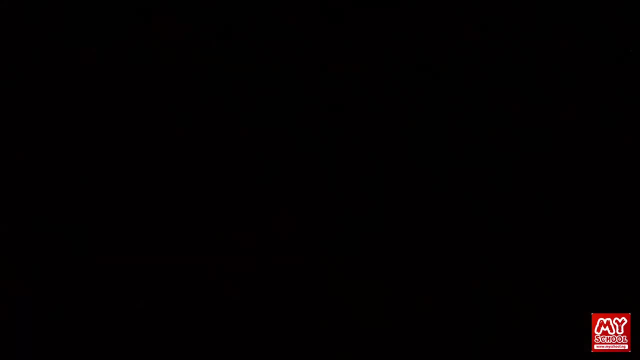 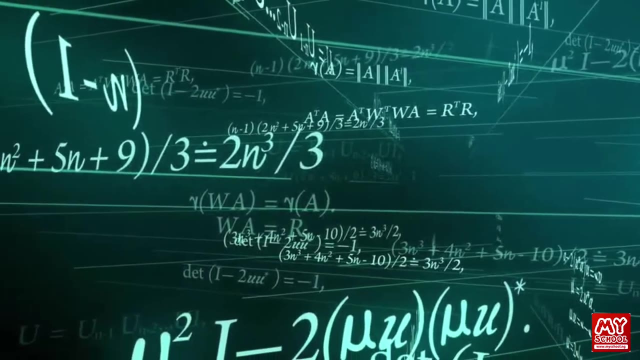 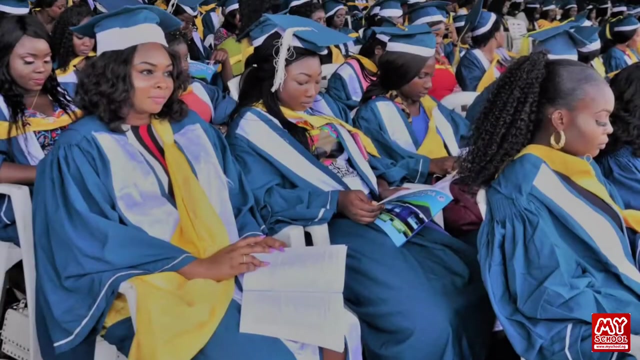 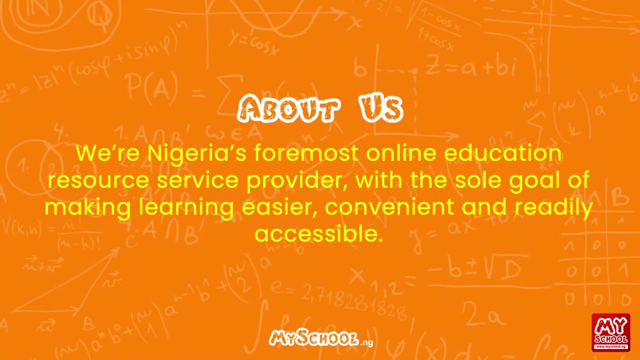 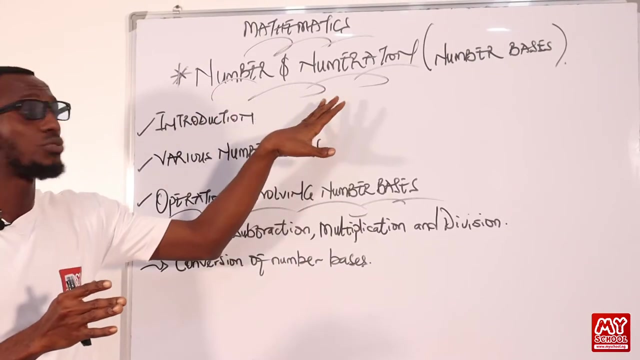 the topic number basis. So all you just need to do is to stay with me as we move to our solution platform to solve the topic number basis. So join me as we move on. So for the first unit, we have topics that have been compressed into it. That's the first unit. 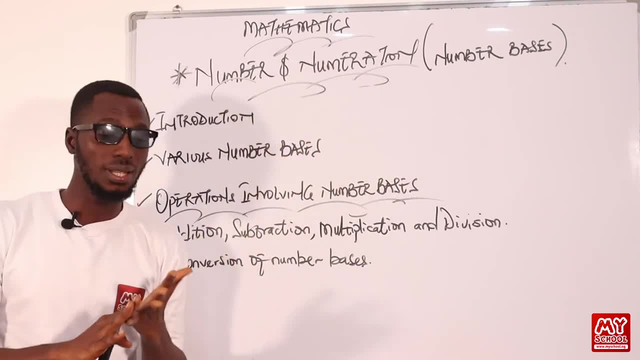 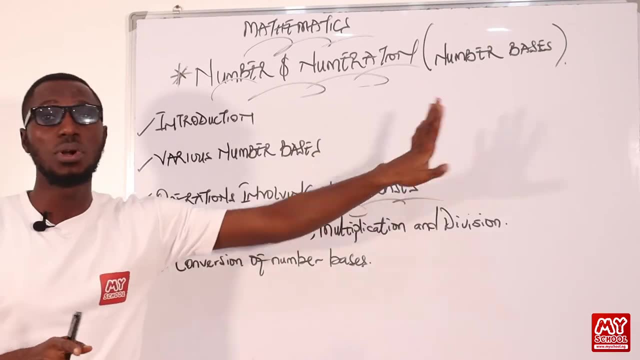 which is number enumeration. We talked about sets that set. here We talk about sorts, We talk about indices and logarithms, We talk about variations. We talk about number basis as well with some other topics. So at first we are considering number basis in the first unit, number enumeration. 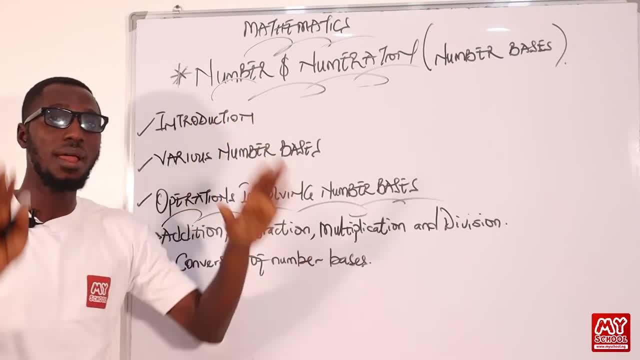 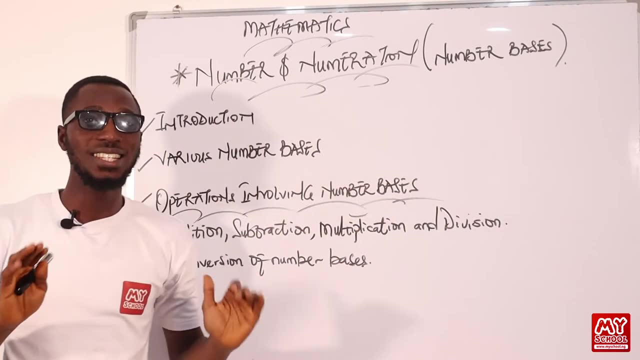 the subject mathematics. So let's just have the hierarchy this way: Mathematics, first unit, number enumeration. In the first unit we are looking at the topic number basis. So let's get introduced to number basis properly, The introduction. what is a number basis You? 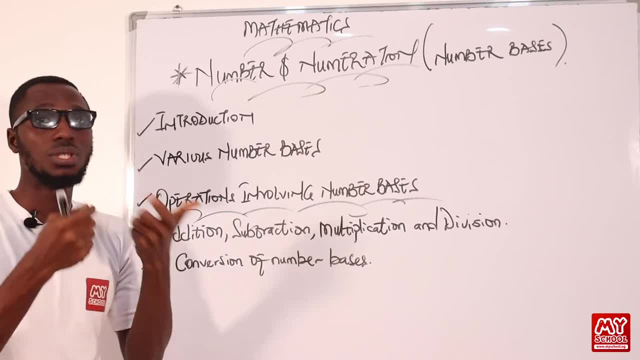 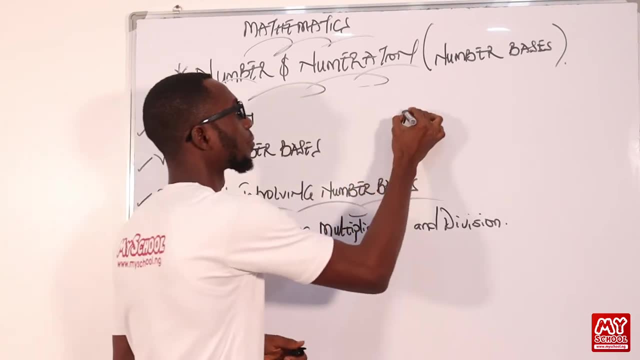 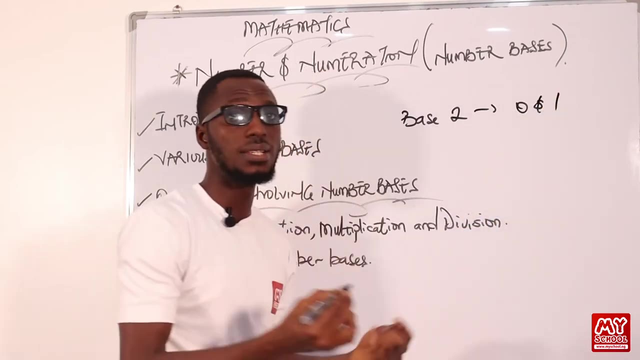 are talking about a counting system that uses a notation to tell you or to represent digits. Okay, this is just what I mean in simple terms When I talk about base two: that tells you there are two different notations, which include zero and one. When I say base three, 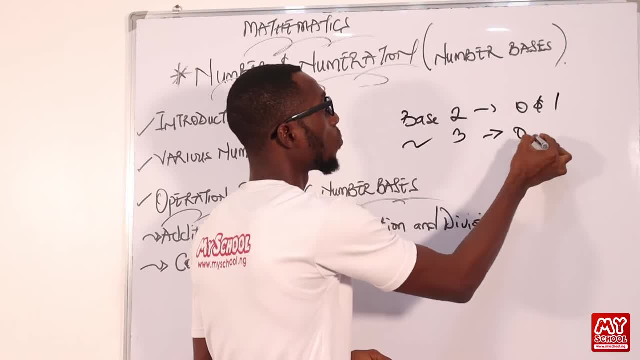 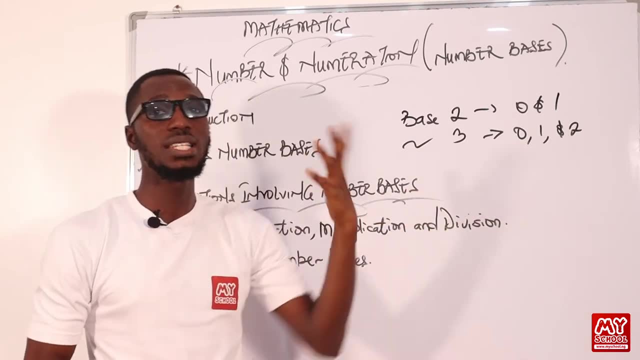 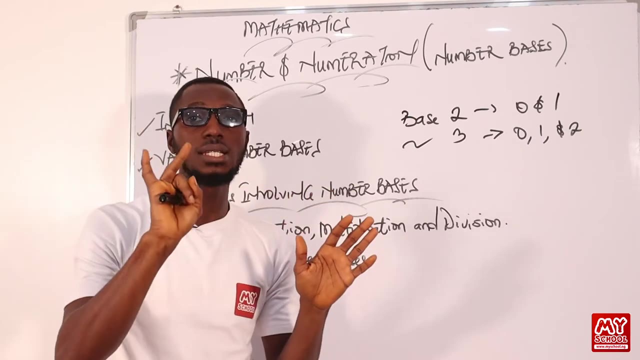 three. that tells you about three different notations: Zero one, two and zero one and two. Okay, that tells us three different notations. When I say base 10, that tells us there are 10 different notations. That is zero one, two, three, four, five, six, seven, eight, nine. Okay, so you can. 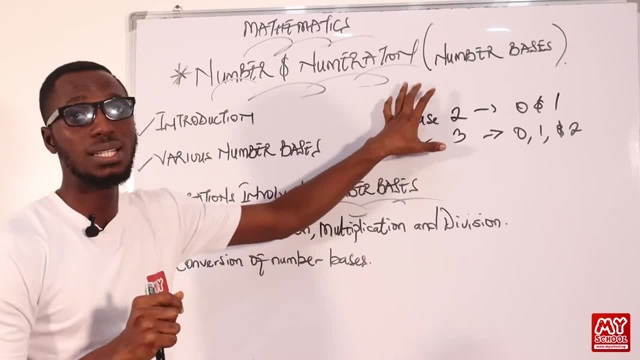 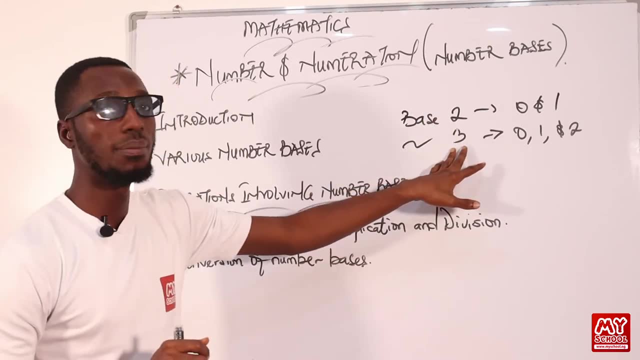 notice a particular trend: that for every base that we are working in, the IS number is minus one less than the base. Okay, so like, for instance, you can see base three, you can see that the IS number is minus one less than the base, So three. 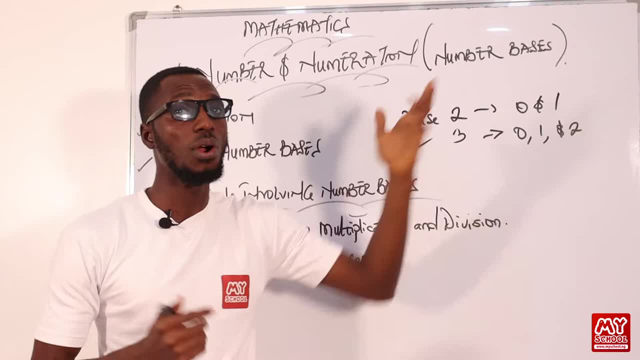 minus one, that is two. Two minus one, that is one. Okay, if we are working in base five, that tells you that the IS number will be four. Now let's take this, for instance, if we are working in base. 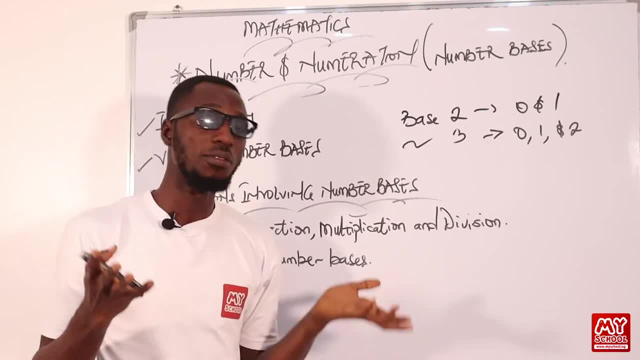 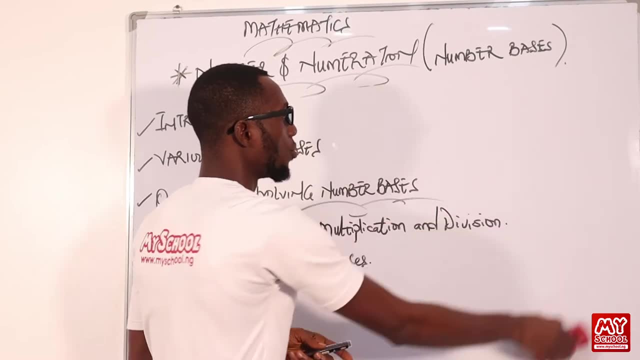 seven. what will be the IS number or IS notation? Of course that will be six. So that is just the brief introduction we have. when it comes to number basis, I can have this as well. You know: number basis. this is how, if I have this compilation, 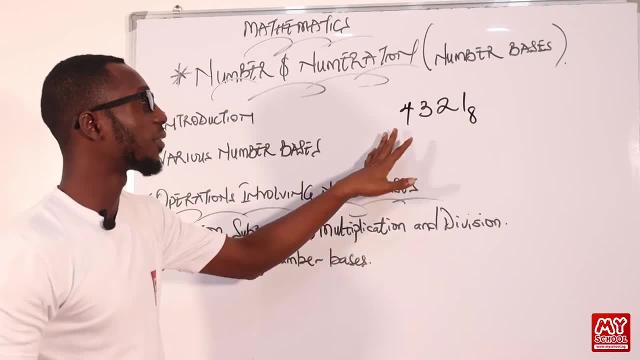 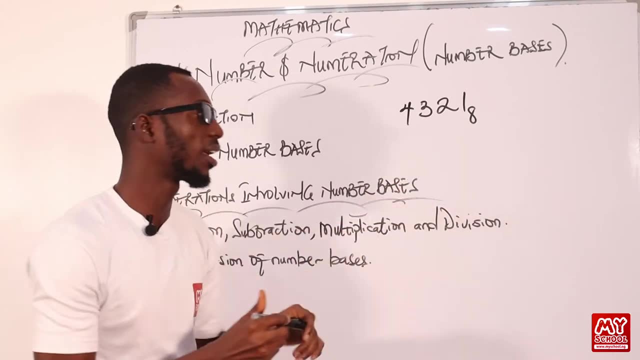 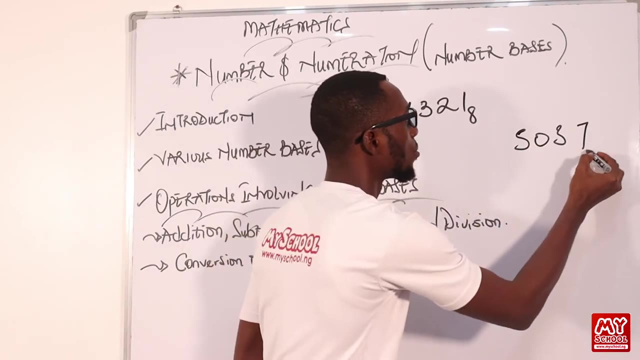 all right. Okay, this is how we read it, Not 4,321.. We don't need to do that in number basis. We just say four, three, two, one base eight. Okay, we can have this. This is 5,037.. Whatever base I want to use, let me say base nine, Okay, so you can see all of this. 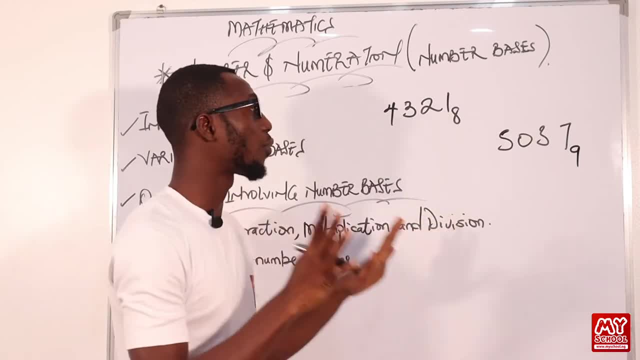 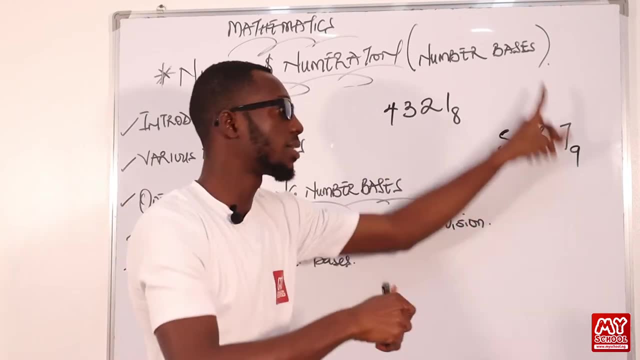 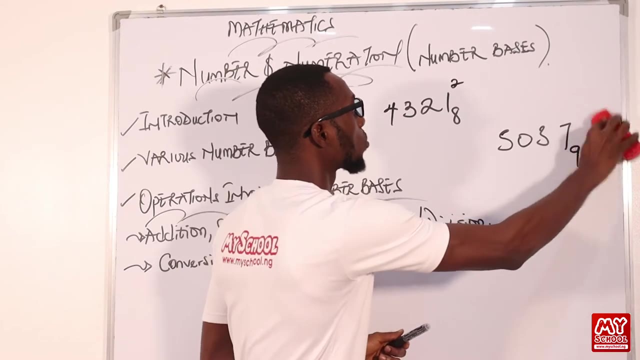 being put together. Then there are some recommendations that will avoid confusion, because they are written as subscripts. You can see underneath, This is superscripts. This is superscripts. Okay, this is subscripts. So you can see. the basis are written as subscripts. So 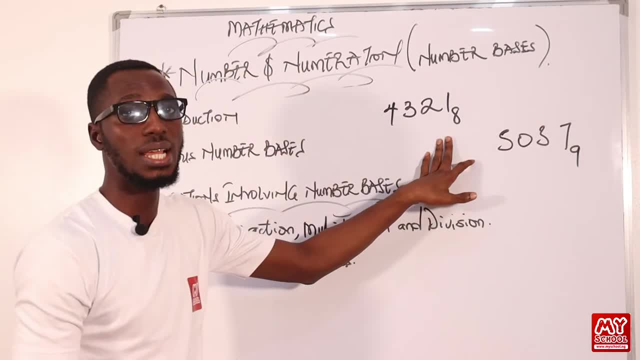 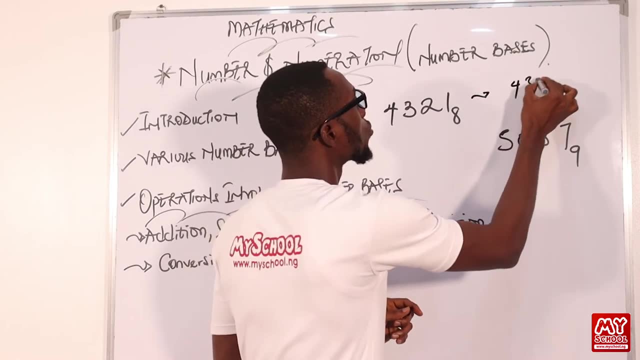 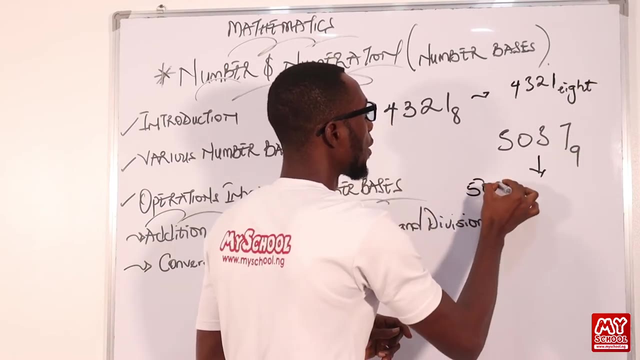 some recommend that, instead of you using digits to represent the basis, to avoid confusion with the value you are given, you can use words instead. So I can have this as 4,321, base eight And this as 5,037, base nine. Okay, so I can have this as 4,321, base eight And this as 5,037,. 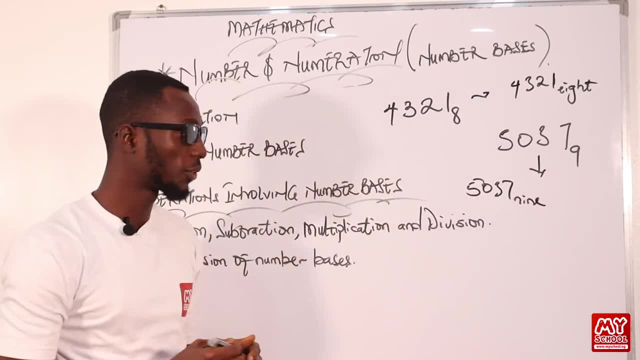 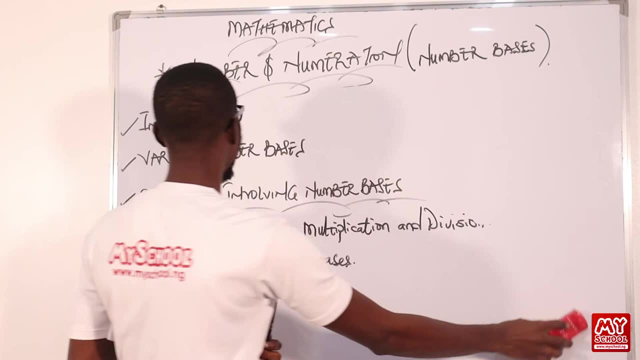 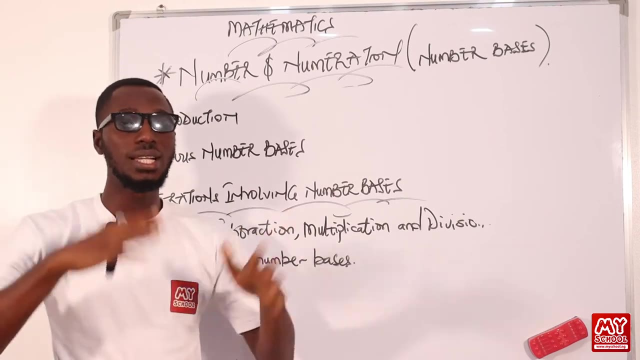 base nine. Okay, just to avoid mix up. So that is a very good introduction to number basis. So let's go into the various number basis that we have. I've just mentioned that we have base two, We have base three, base four, five, six, seven, eight and what have you? So base: 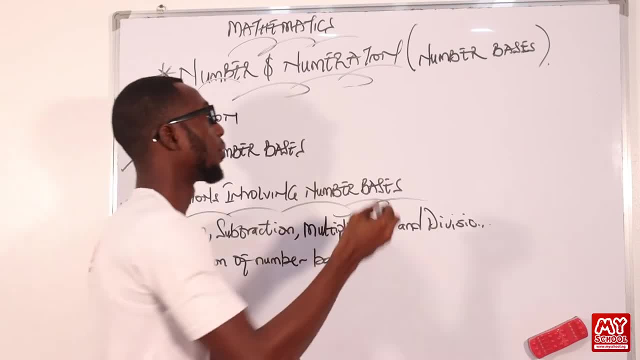 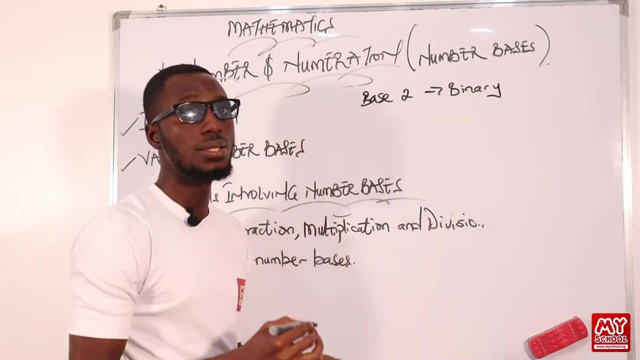 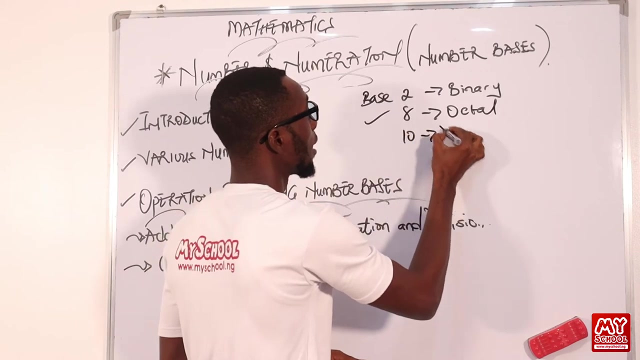 two. you can refer to base two as your binary system. Okay, base two, This is binary. All right, Your base eight, that is your octal. Your base ten, that is your decimal, Or you can use your, or you can call it the denary. Then base 16, we have your hexadecimal. 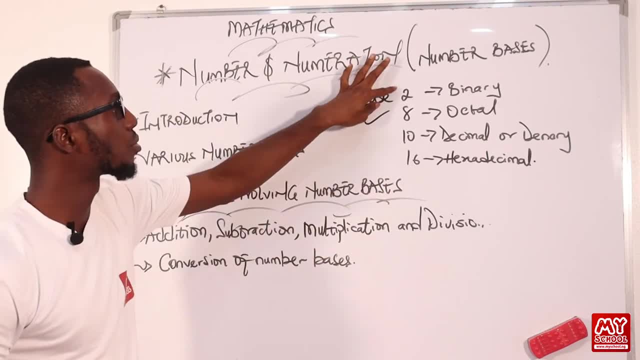 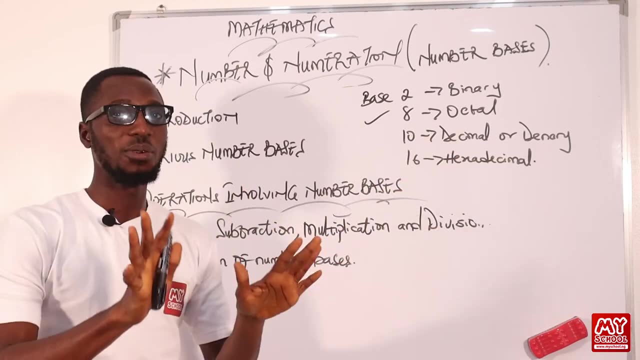 Okay so, and of course we can pull a linkage between base two, base eight and base ten. Okay so, that's where we look at the four bits. the three bits complement, But we're not going there right now. Okay so you can see your base two, your base eight, your base ten. 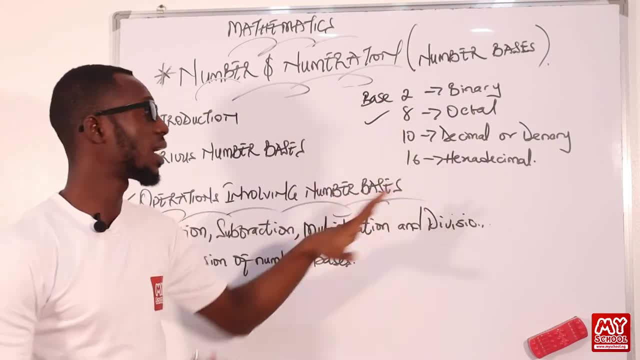 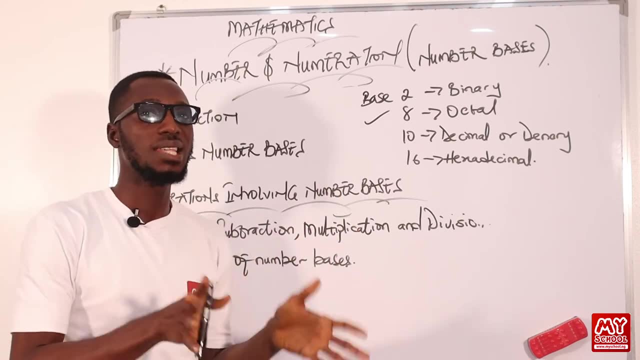 base 16.. Of course there are other bases, but these are the important ones. And I just want us to know this: The normal addition, subtraction, division, multiplication that we do, we do them in base ten. That is why, when you are trying to do some simple takeaway, you realize that by the 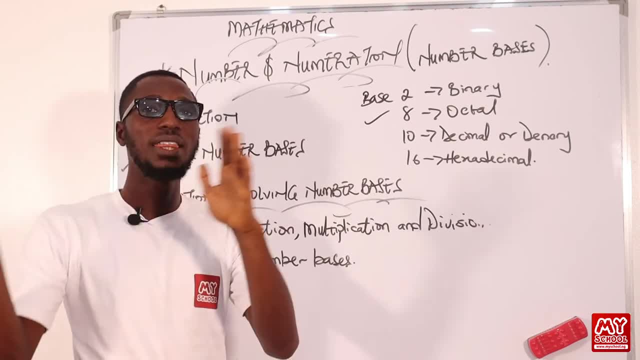 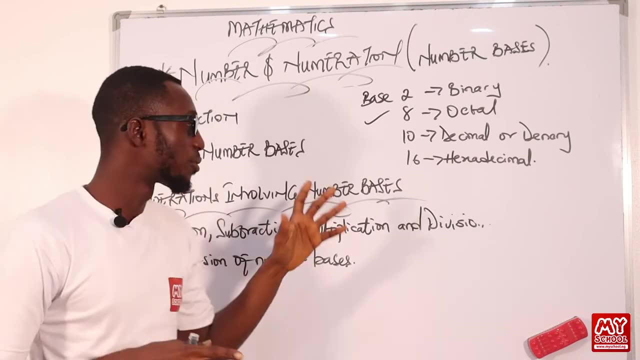 time you are borrowing from the next neighbor. okay, you see that, whatever thing you are adding, we had it by ten. So your natural base we've been working on working with so far is base ten. So join me as we move to the next part of this topic. 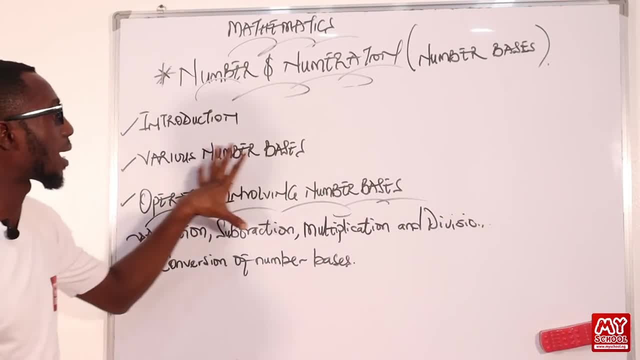 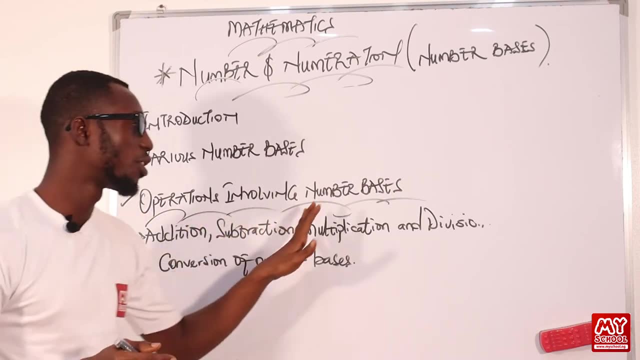 number basis. We are looking at the different operations that are involved or that have been engaged in number basis. So those operations are just like your addition, your subtraction, your multiplication and your division. It's important to know that you can just carry these. 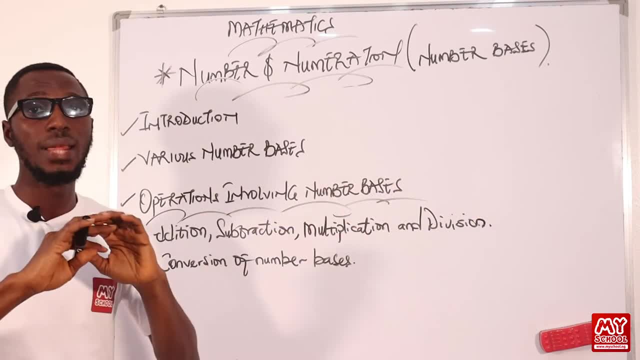 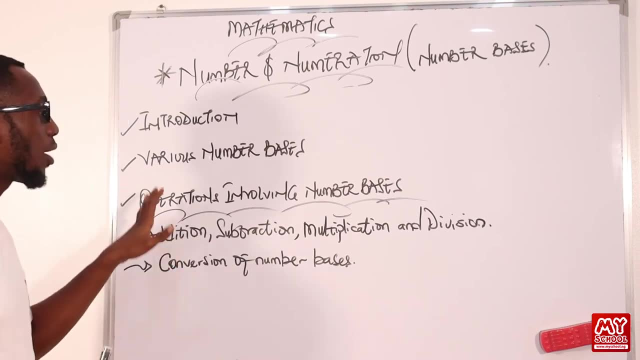 operations out just the way you used to do your regular division, multiplication, addition. There are just some simple rules that you have to take note of, okay, So when it comes to operating in addition, or subtraction or multiplication- let me take, for instance, subtraction- If I'm 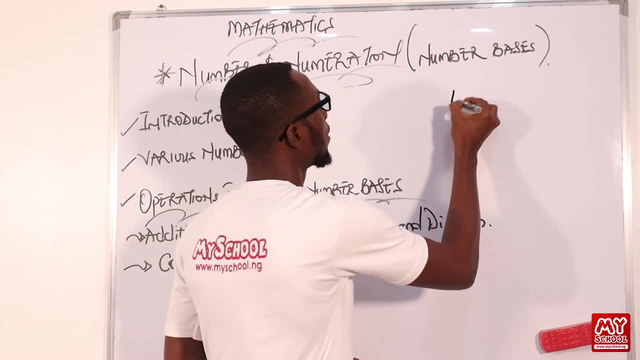 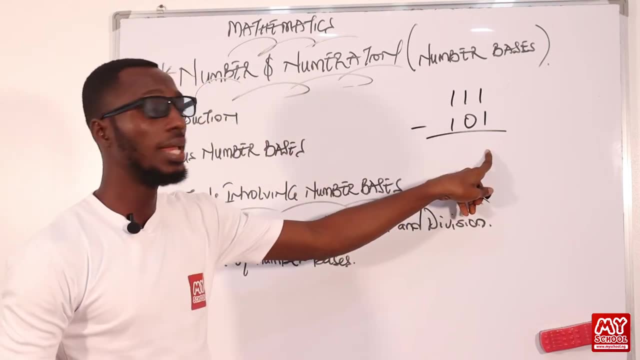 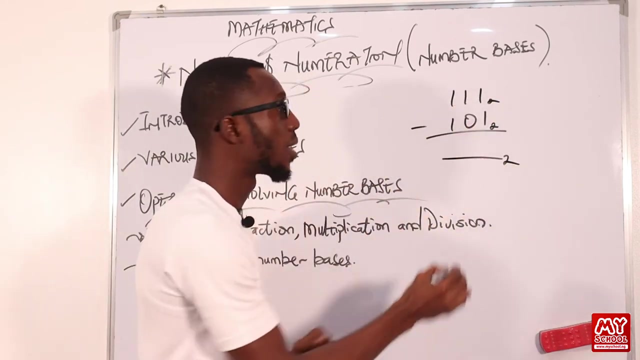 asked to subtract in base two, for instance, I have something like this: Okay, All right, So in this case I can decide to use the regular way to work around this: Right One minus one, that is, zero One minus. 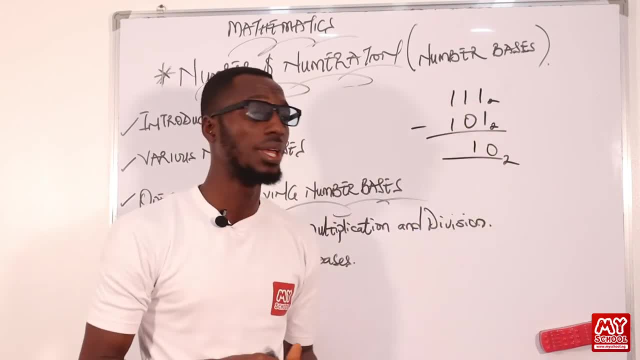 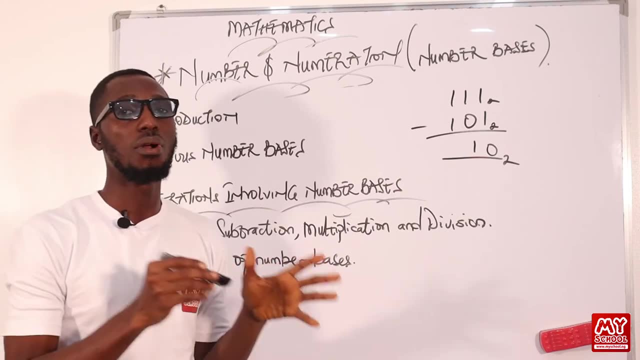 zero. that is one. one minus one, that is zero. okay, i can decide to do it this way, or i can decide to use what we know as the one complement and the two complements. okay, one complement and the two complement. i'm going to be sharing that with you in the next video. that is where we have the full 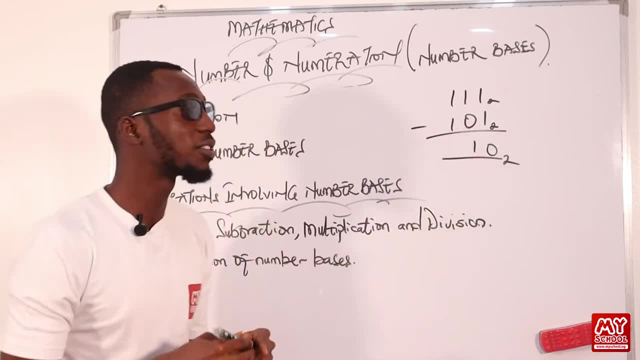 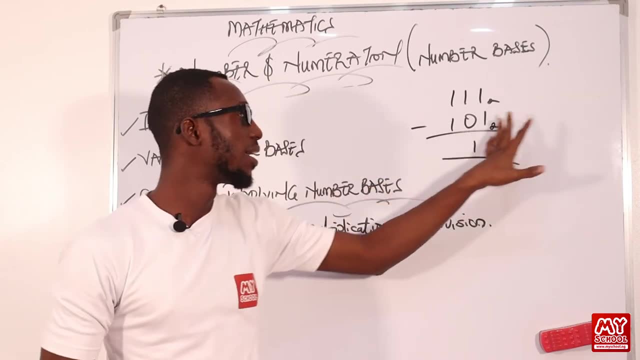 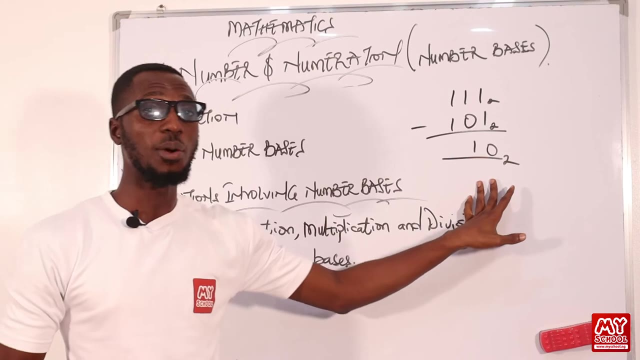 compilation. okay, so or i can decide to first convert this to their various um representation or various values in base 10. this to base 10, then i will now do the normal subtraction, then bring the answer back to the base 2 that we are working in. don't worry, in the next video i will provide. 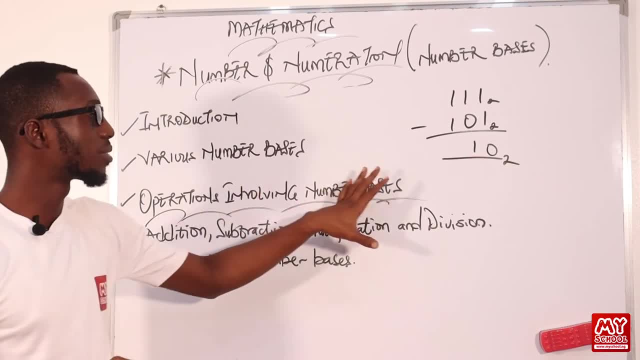 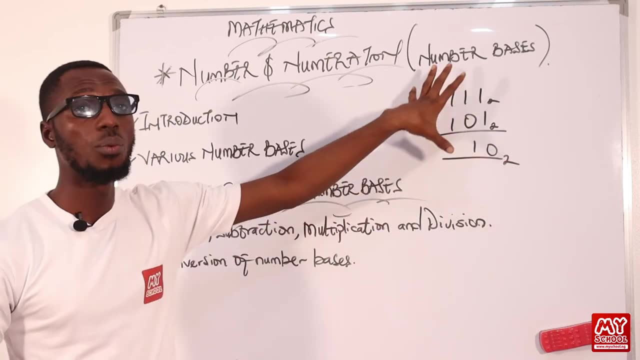 you with more step-by-step explanation so we can decide to use this. if we are working in base 10, we can use another method. we can use in regular subtraction or regular addition, but if you are working, uh, on subtraction in base 10, instead of using the one complement and the two complements, 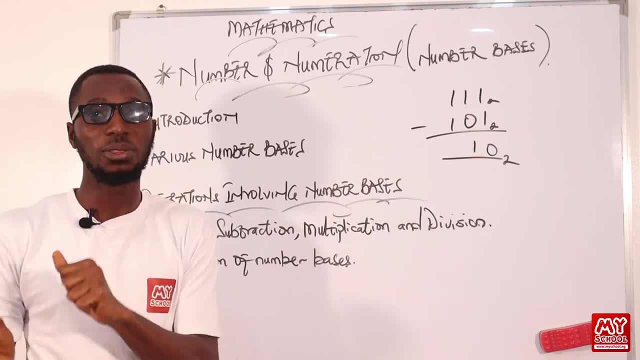 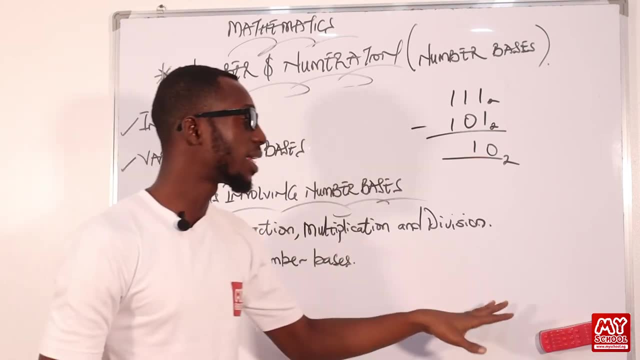 you'll be using the nine complements and the ten. you'll be using the nine complements and the ten complements and the ten complements complement method. don't worry, i will share that with you, okay, so then we have conversion from one base to the other. so like, for instance, i want to convert from. let's say, i want to convert this. 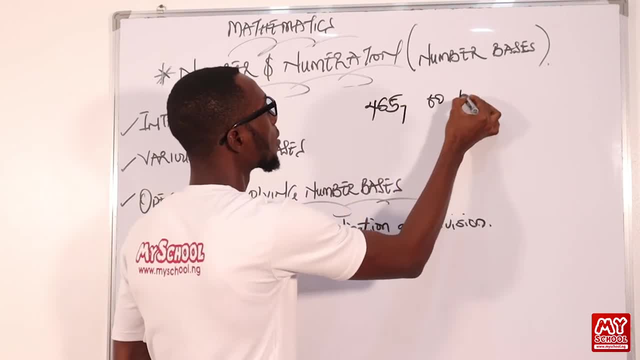 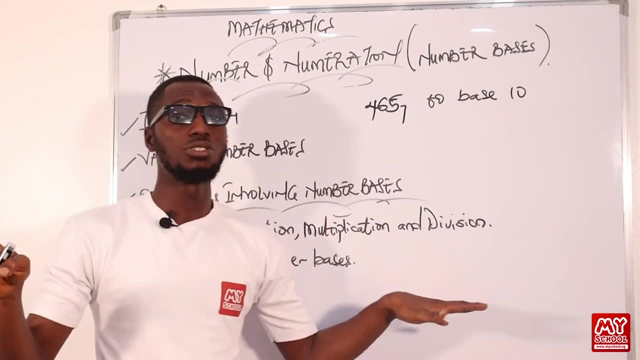 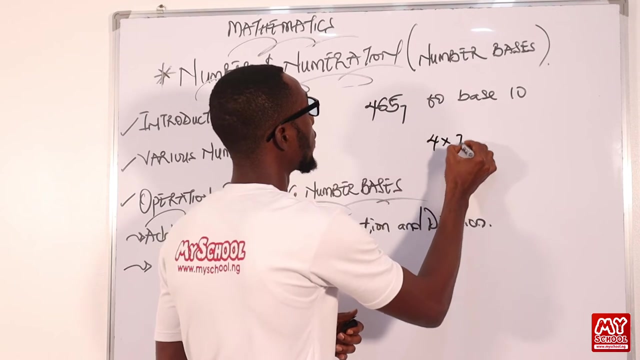 four, six, five be seven to base ten. okay, so i can use different method. i can use the normal expansion method or i we can call it the power expansion, all right, so this is what i mean. that was just before: four times seven raised to power two plus six times seven raised to power one plus five times. 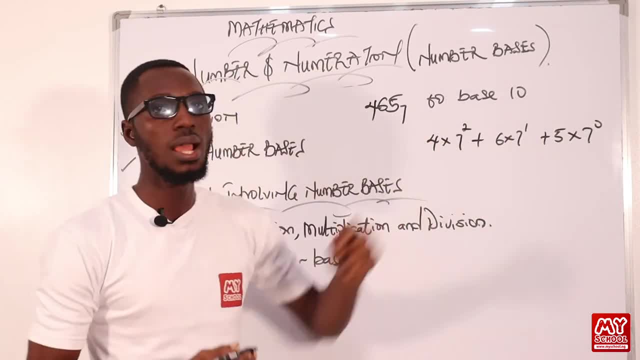 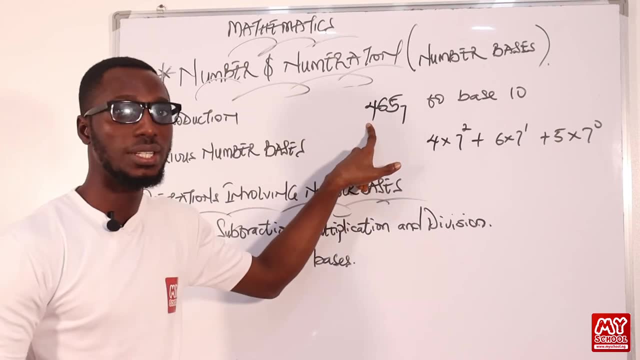 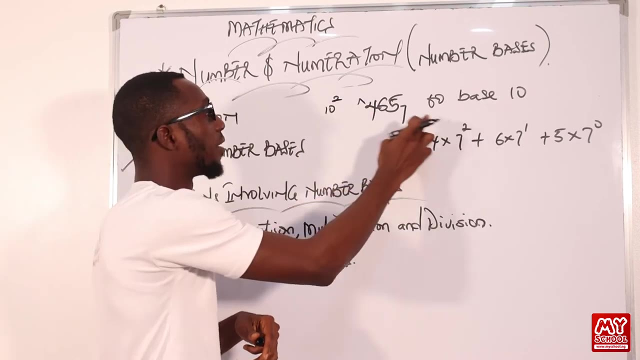 seven raised to power zero. i know you may wonder how we have all these powers. it's just very easy. just introduce your knowledge of place values. okay, this is unit things and hundred, so remember that this is hundred. hundred means ten raised to power two, isn't it? that is the two we have here. 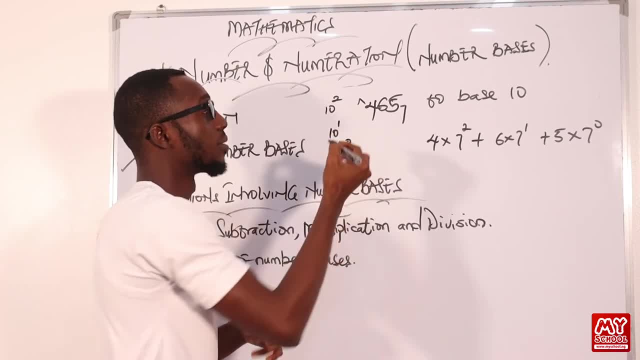 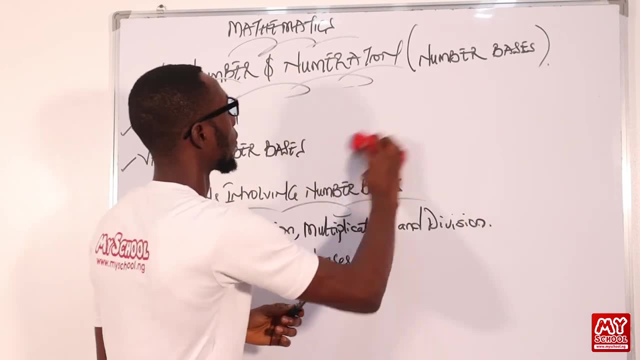 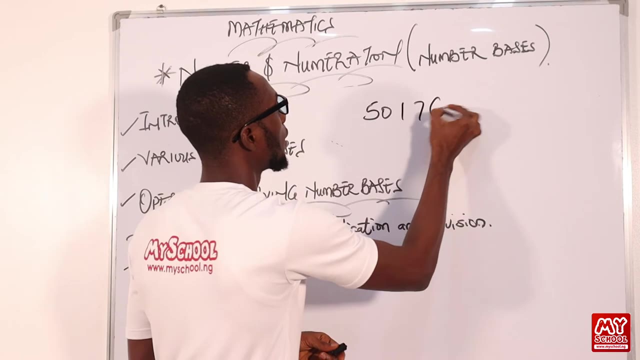 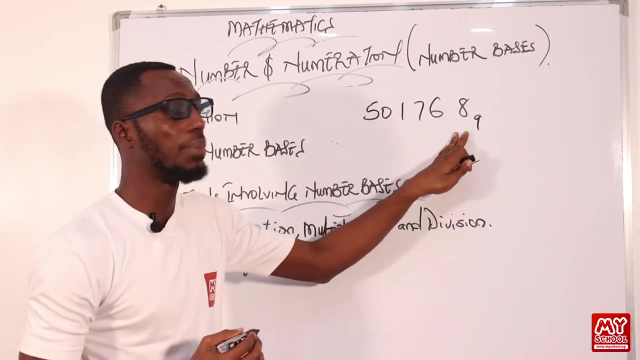 tens means ten raised to power one, then you need ten raised to power zero. very easy, right. so if i have something like this, if i have probably i have something like this: five, zero, one, seven, six, eight. so let me say base nine. okay, you can see, i'm very um cautious about the base i'm introducing. see, the is we can have. 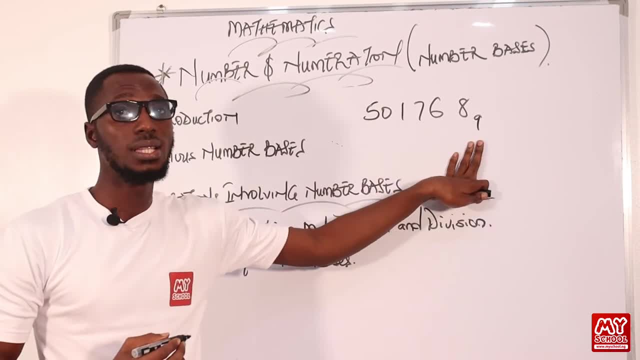 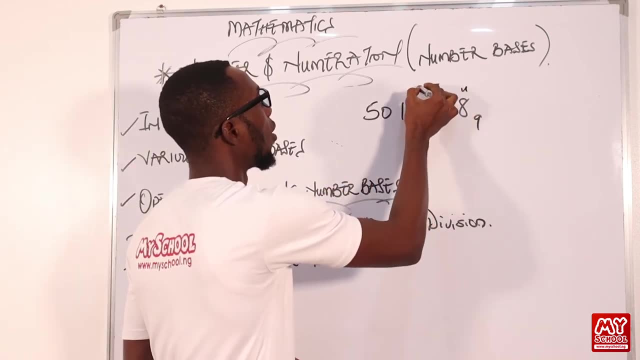 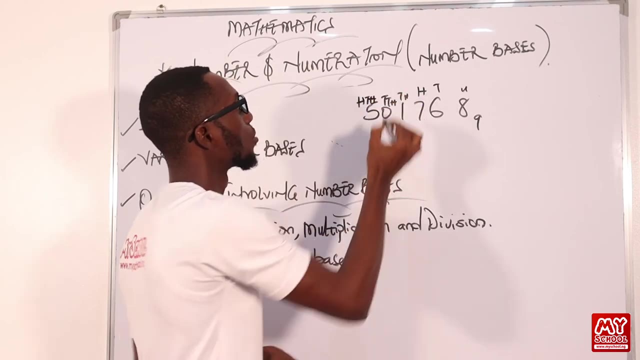 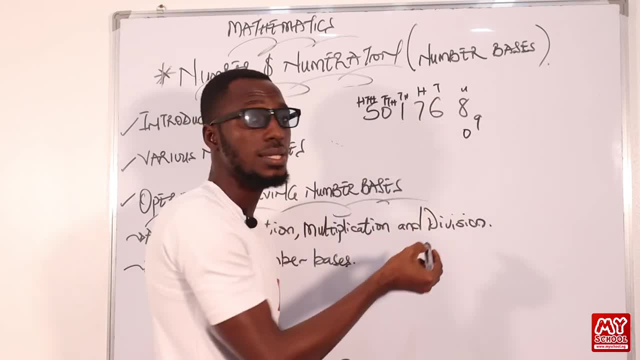 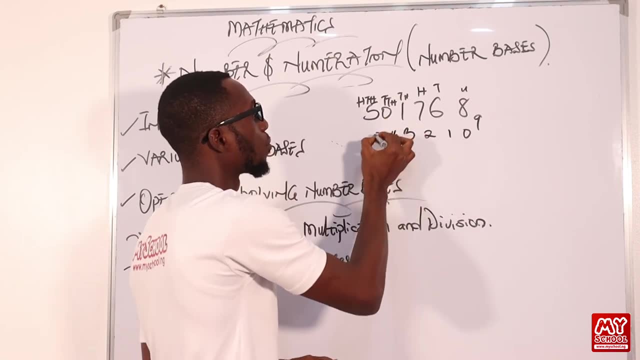 your unit is ten raised to power zero. right, your tens is ten raised to power one hundred. ten raised to power two. this turns to power three, this ten is to power four and this ten raised to power five. so if i'm introducing or using the expansion method, what i would just do, starting with the 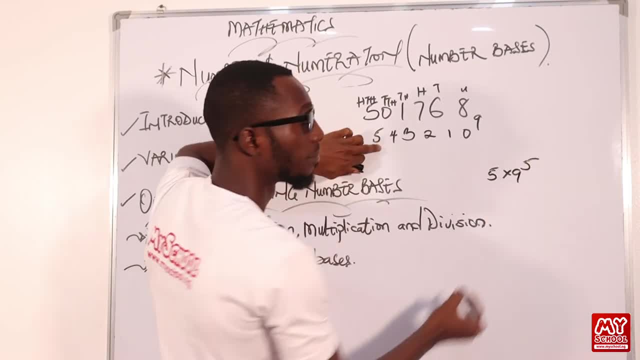 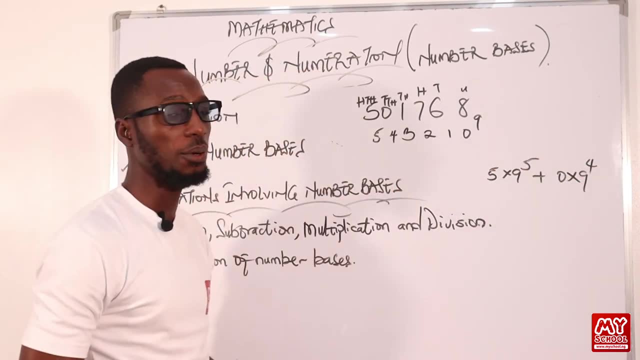 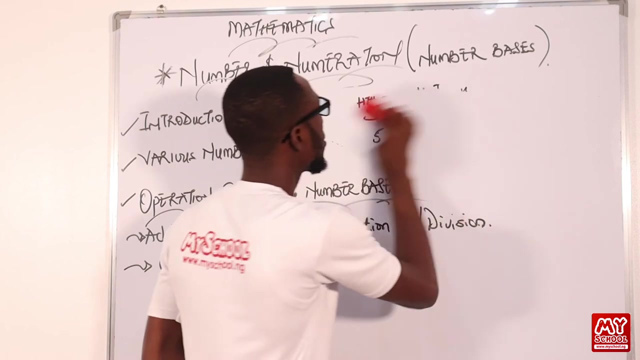 first one: five times nine, raised to power five. right, then this plus zero times nine, raised to power four, just like that. okay, so that is where we got all these powers that are being introduced to work on this set of operations. so that is what we'll be.